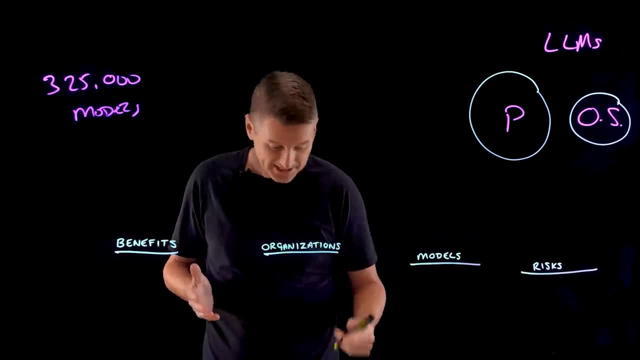 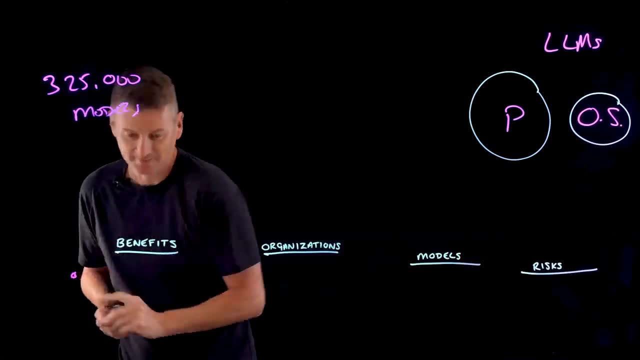 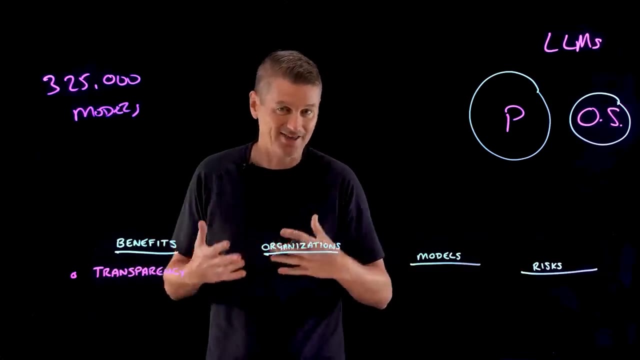 the risks associated with using them. Now, clearly, one of the benefits of a open source large language model that has to be transparency. Open source LLMs may offer better insights: insight into how they work, their architecture and the training data used to develop them. 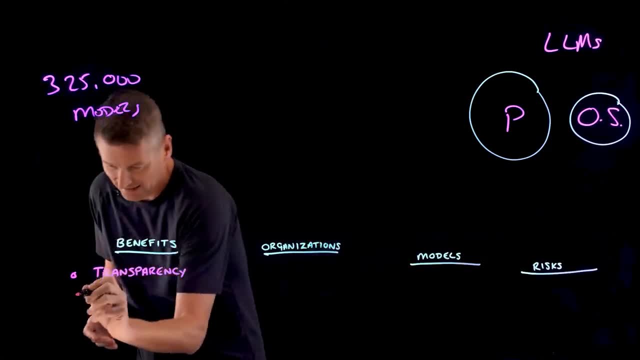 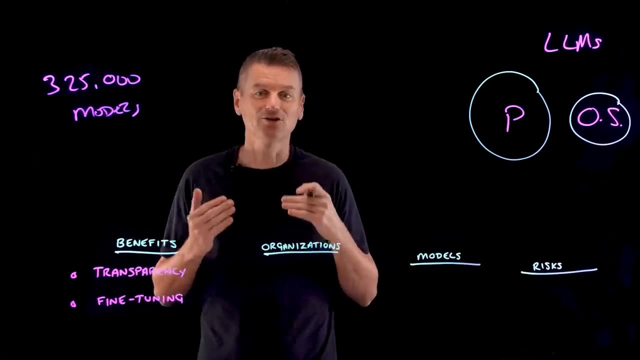 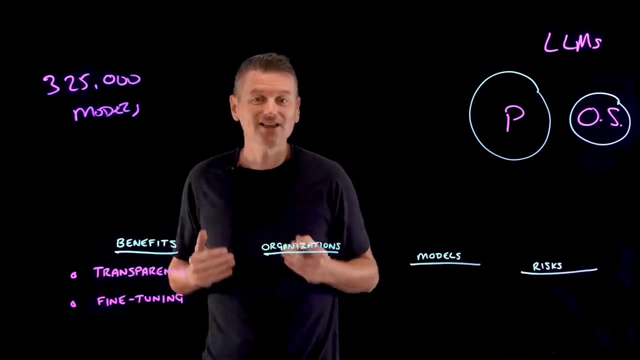 Another big one is pre-trained open source LLMs allow a process called fine tuning. That means you can add features to the LLM that benefit your specific use case, and the LLMs can be trained on specific data sets. So I can fine tune an LLM with my own data And 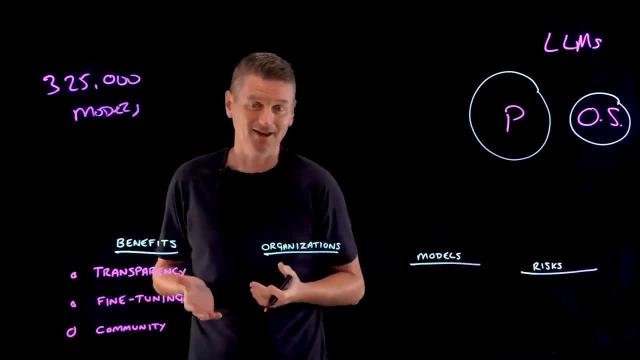 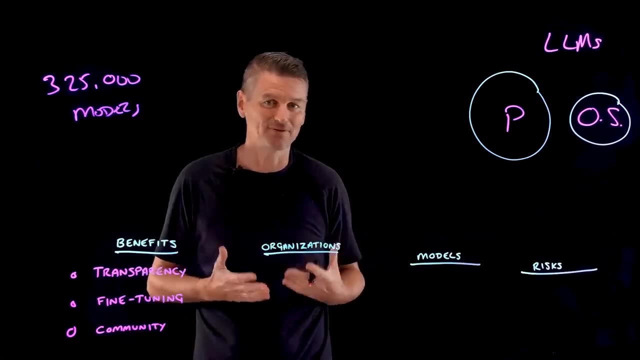 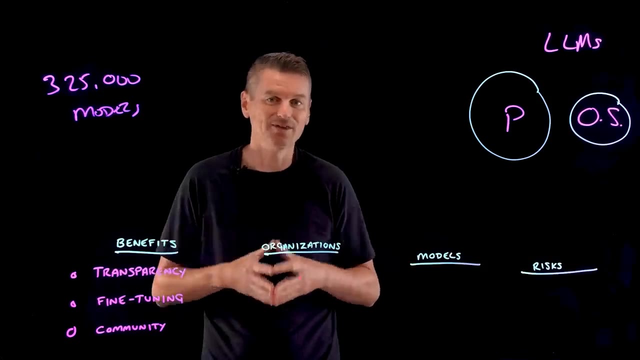 now we are talking about the importance of open source LLMs. Let's talk about a different aspect of open source LLMs that is interlinked with many other programs. The way open source LLMs are more dynamic. they offer an überall service. 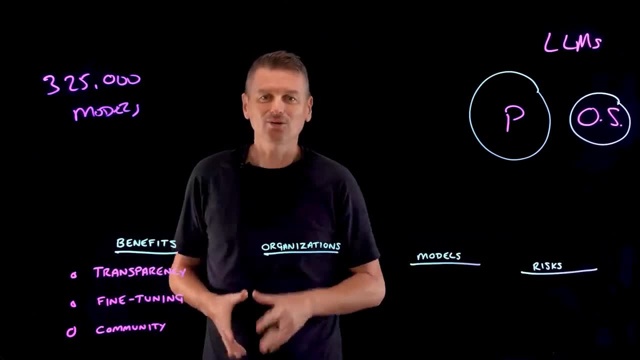 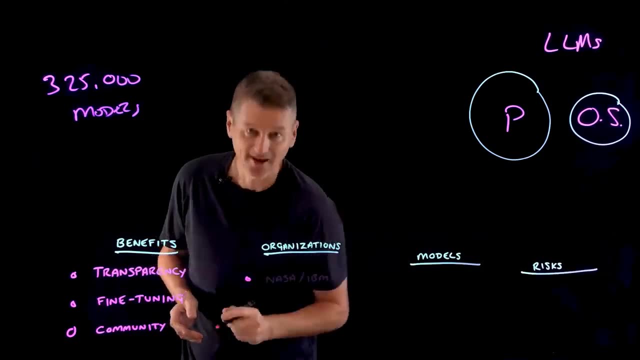 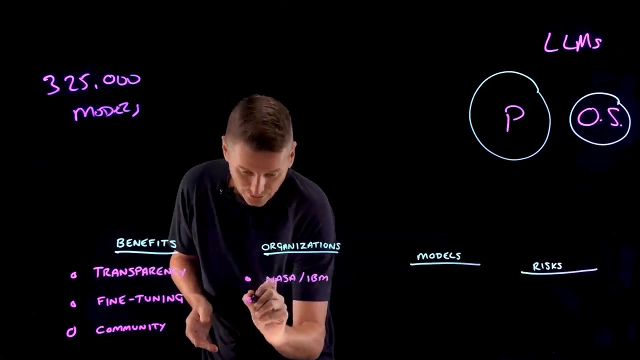 on buyers with a full market share of their products in an attractive quarter. When metals ales are traded in the UK, with their market share decreasing, they provide quite a high, And IBM developed an open-source LLM trained on geospatial data. Some healthcare organizations use open-source LLMs for diagnostic tools and treatment optimizations. 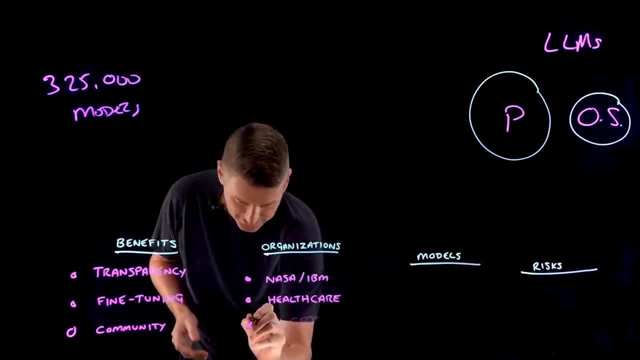 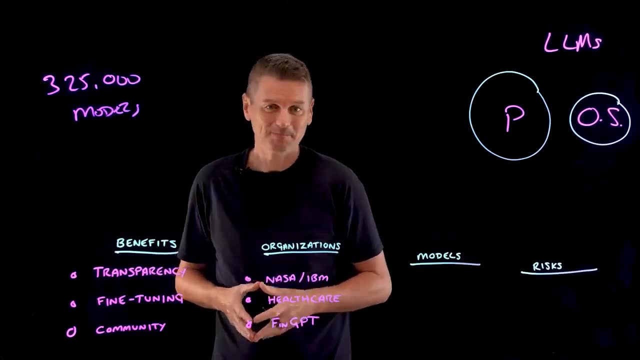 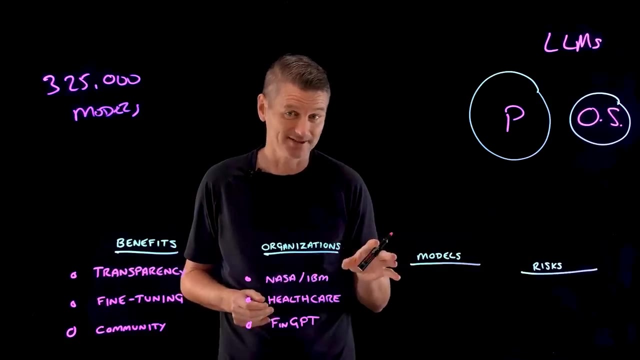 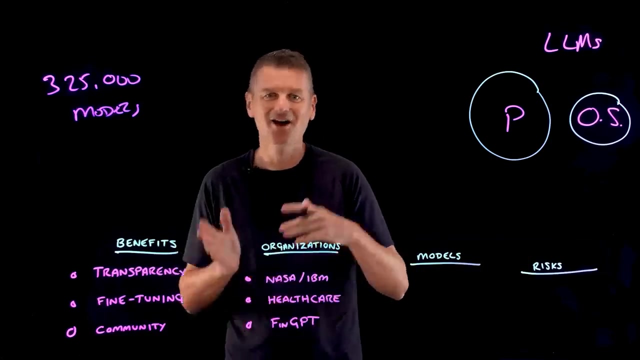 There's an open-source LLM called FinGPT Fin financial. it was developed for the financial industry, Which brings us on to the topic of talking about some specific open-source LLMs that you might find of interest Now. Hugging Face maintains an open LLM leaderboard and that tracks, ranks and evaluates open-source LLMs on various benchmarks. 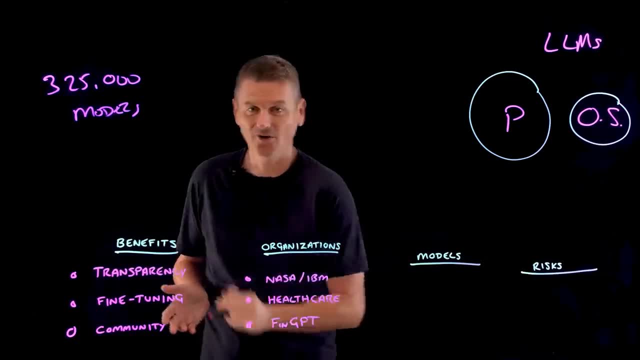 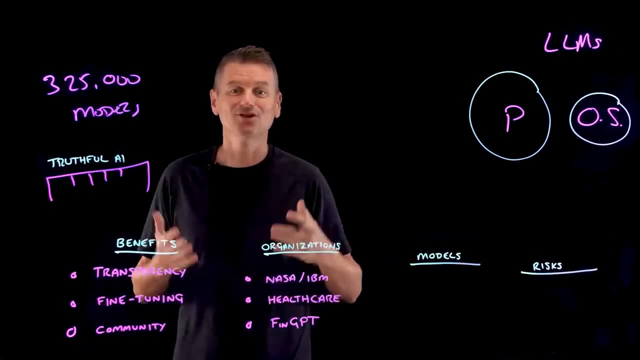 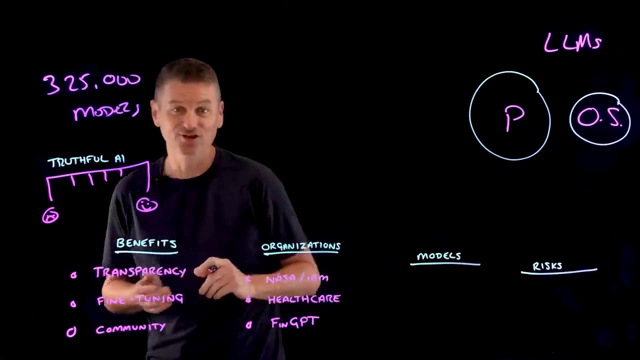 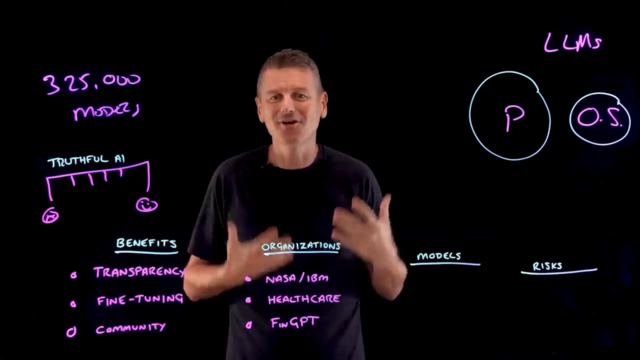 Like which LLM is scoring highest on the Truthful AI benchmark series, which measures whether a language model is truthful in generating answers to questions, so it gives those answers a score And the top spots on this leaderboard. they change frequently and it's quite fun to watch the progress these models are making.